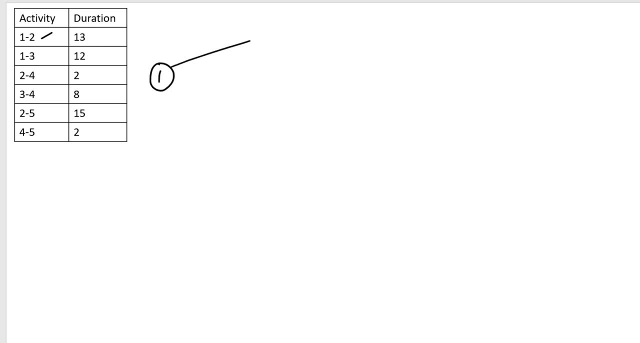 the very first level. let me start from one to activity two. From node one, there is another, activity three. Then, in order to start the fourth activity, we should have completed second activity as well as third activity, Fourth node. here, two to four, we are. 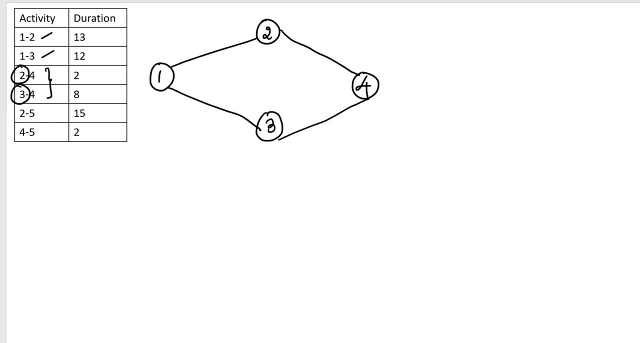 connecting, and three to four we are connecting Again. for the fifth activity to start, we should have completed second activity and we should have completed fourth activity. So let's see fifth activity from two to five. then we have four to five. 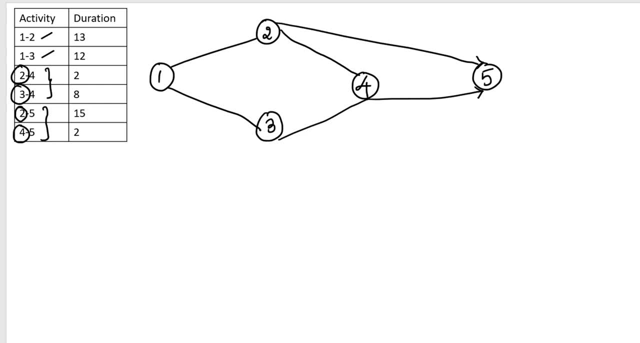 So now that we have done the network construction, let's go and fill the duration. for the activity one to two, it's 13.. For the activity one to three, it's 12.. For the activity two to four, it's going to be two. For the activity three to four, it's eight. For the activity: 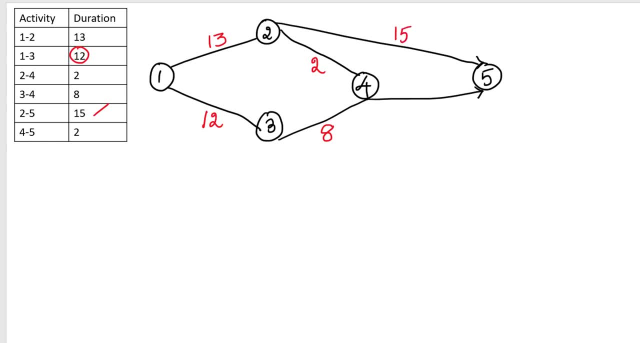 two to five, it's 15.. And for the activity, four to five, it's two. Now that we have completed the network construction, construction, let's identify the different path that is available to us. at the first level, we have gotten the first path: 1 to 2 and 2 to 5. at the second level, we have gotten 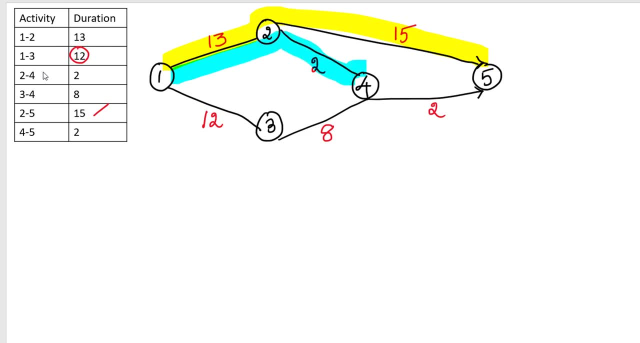 1 to 2, 2 to 4, then 4 to 5 activity at the third level we have gotten 1 to 3, 3 to 4 and 4 to 5, three different path we have now let's calculate the duration of every path. 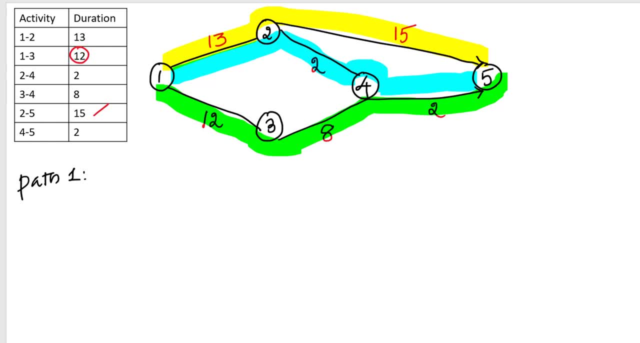 path one. focus on the yellow color. it's between 1 to 2 and 2 to 5, and what's the duration of 1 to 2? 13 plus 2 to 5 is 15.. so we have gotten 28 weeks. let's move on to path 2. 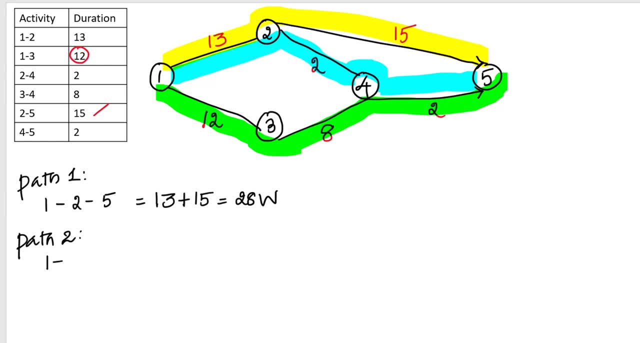 path 2 focus on the blue color: 1 to 2, then 2 to 4, then 4 to 5. so which will give us: 1 to 2 is 13 weeks, plus 2 to 4 is 2 weeks, plus 4 to 5 is 2 weeks time. so which will give us: 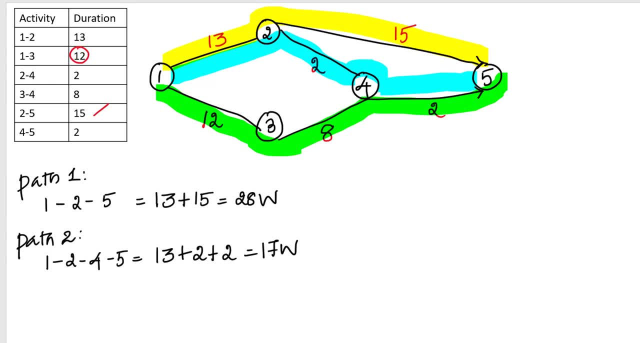 17 weeks. let's calculate path 3, 1 to 3, 3 to 4 and 4 to 5, so the duration of 1 to 3 is 12.. the duration of 3 to 4 is 8 and the duration of 4 to 5 is 2, so which will give us 22 weeks. 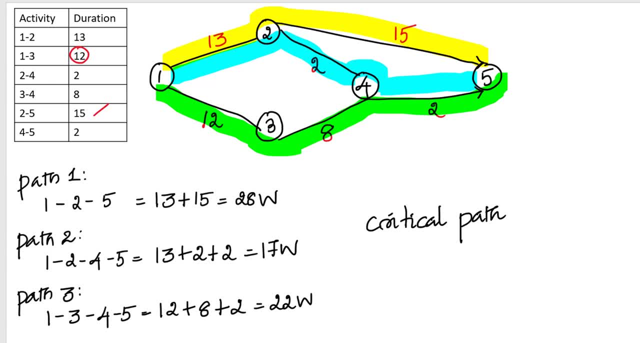 for identifying the critical path. we take the maximum of the duration. let's look at the value and take the maximum. one max of path 1 is 2 weeks, 28, path 2 is 17 and path 3 is 22.. the maximum is 28 weeks. 28 weeks is path 1. 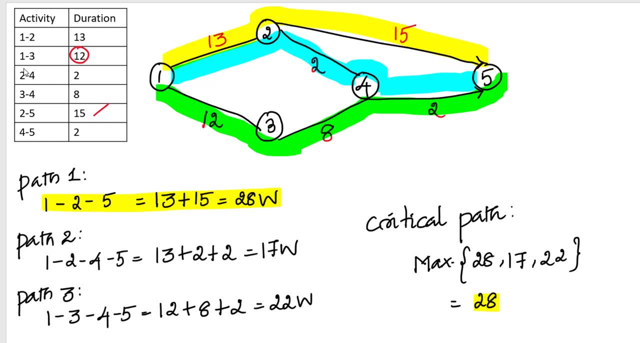 we will consider the path 1 to 2 and 2 to 5 as the critical path. so now that we have done the network diagram and at the next level we have identified the critical path, now let's go and calculate. what are the early start time, early finish time and late? 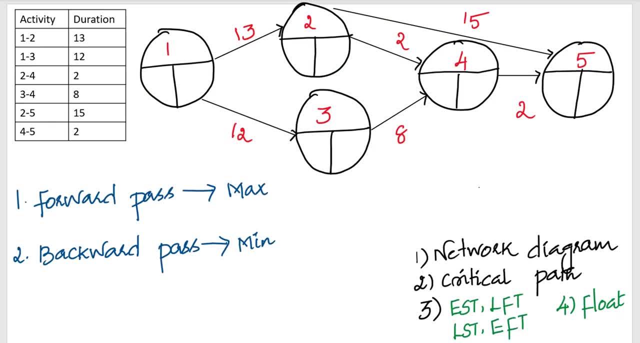 start time and late finish time. Now that we have already calculated the network diagram and identified the critical path, at the next level we have to identify the activity time. So in order to do that, what I have done in our basic network diagram, i have inserted two more boxes to accommodate EST and LFT. 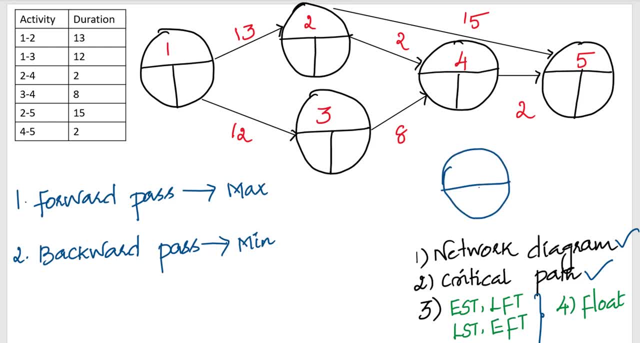 This is the basic diagram that we have gotten. this represents the activity and this is going to represent the early start time and this is going to represent the late finish time and on the arrow, we have taken the duration. This is all. we have done it here. Now let's go and calculate the early start time first. This is early start time and this is 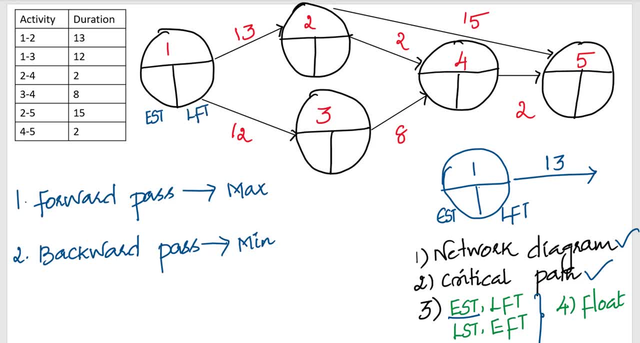 going to be late finish time. Now look at this: whenever we commence any of the activity, especially when it is going from 1 to 2, 1 to 3, then the start time is always 0.. Now take 0 plus 13: we. 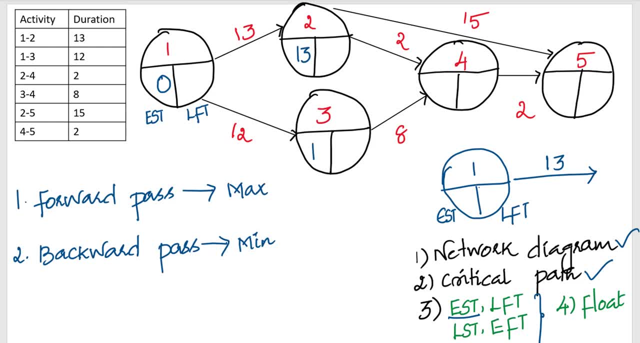 have 13 here. 0 plus 12, we will have 12.. Now let's calculate for the activity 2 to 4.. For the fourth activity we have got two nodes coming from 2 to 4 and 3 to 4.. So 13 plus 2 it's 15 here. 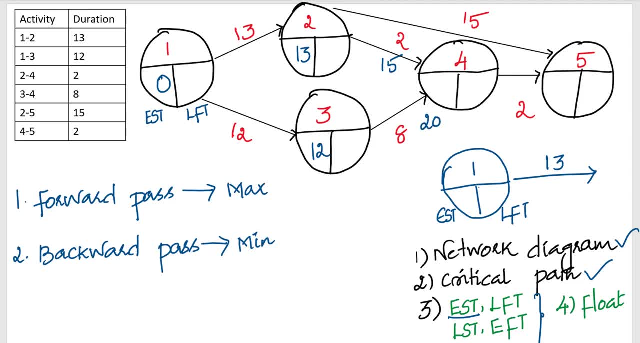 12 plus 8, it's 20 here. Whenever we are doing a forward pass, we always have to take the maximum value. So the maximum is 20. we are making 20 here, 22. i'm marking it outside because, again for the fifth one, we have got another node coming from. 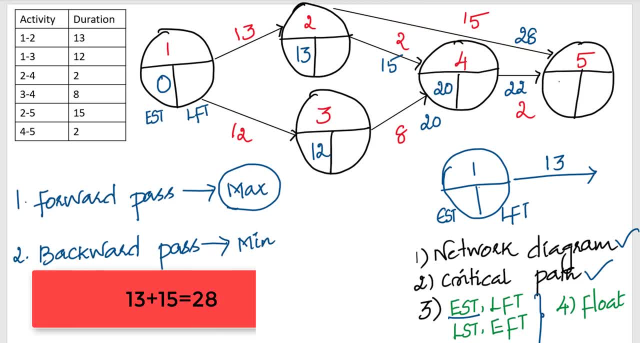 two. the maximum of 28, comma 22 is 28. so we are marking 28 here. the calculation of est is done. now we have to calculate the lft for lft. whatever the duration we have got in here, take the duration as such: 28. now we have to go backwards. 28 minus 2, we will have 26 here. 26 minus 8, we will have 18. 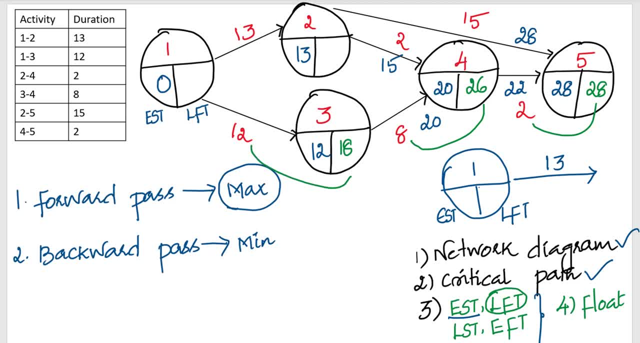 here 18 minus 12, we will have 6 here. i'm marking it outside because we have to calculate for the activity 2 to 1. also, there is two different nodes coming in, so i have put it outside now. once we finish this, then we will take the minimum of that. now look at this. 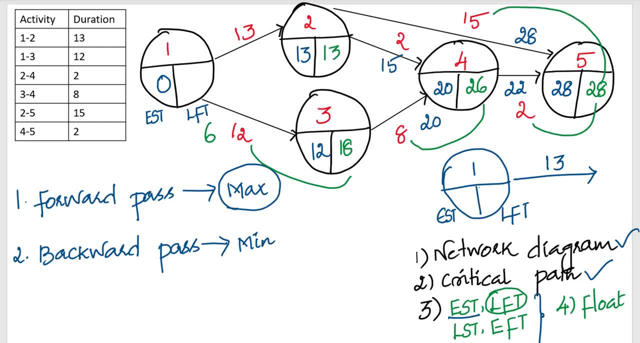 28 minus 15, we have got 13 here. now 13 minus 13, we have gotten 0 here. for the backward pass, it's always the minimum. now, minimum of 0, comma 6 is 0. this is the best way that we can do a. 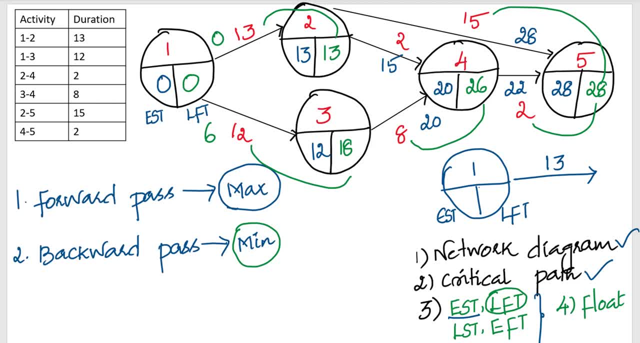 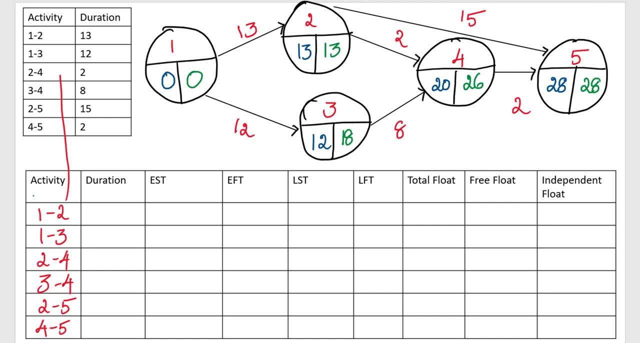 early start time and a late finish time. now let's calculate late start time and early finish time and with the float also, this activity comes from this particular table. in the same way, park the duration also. we have parked in the activity and the duration let's park in the. 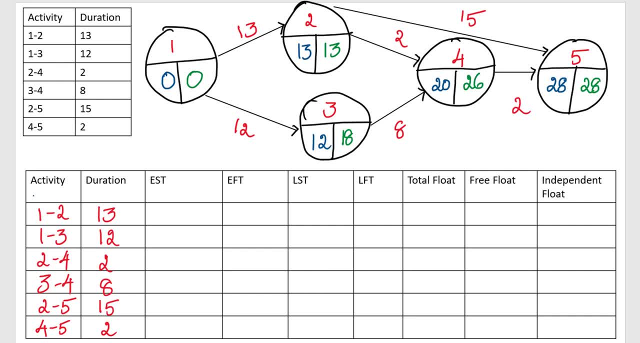 early start time. when you are doing early start time, always look at the node of this activity. only then you will have the right answer. so for the activity 1, the early start time is 0. then again for the activity 1, the early start time is 0. for the activity 2, the early start time is 13. 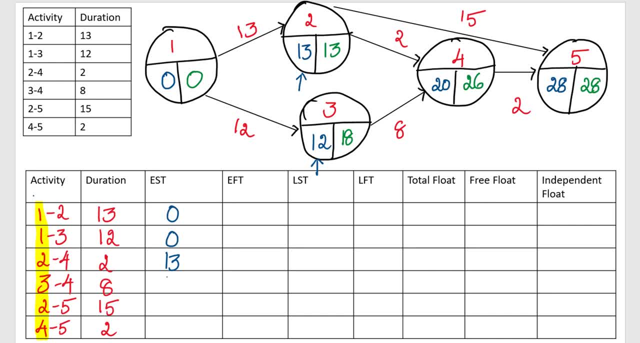 for the activity 3, the early start time is 12.. for the activity 2: again, it's 13. for the activity 4: it's here, it's 20.. when you are doing the lft, always please be assured that you take the end node of it. for the activity 2. 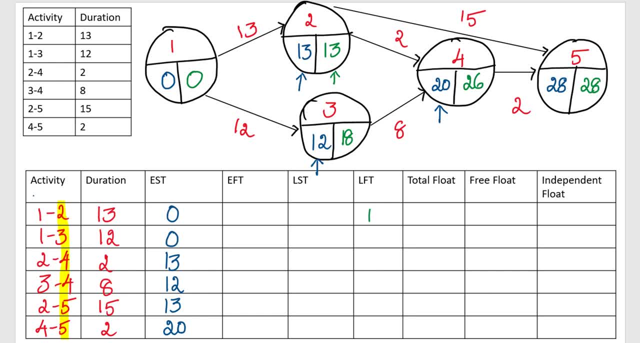 the late finish time is here 13.. then for the activity 3, it's here 18. for the activity 4, it's here 26.. then again we have four. four is 26 again. for the fifth one, it's here 28 again. the next one is also 5, so we are backing in 28. 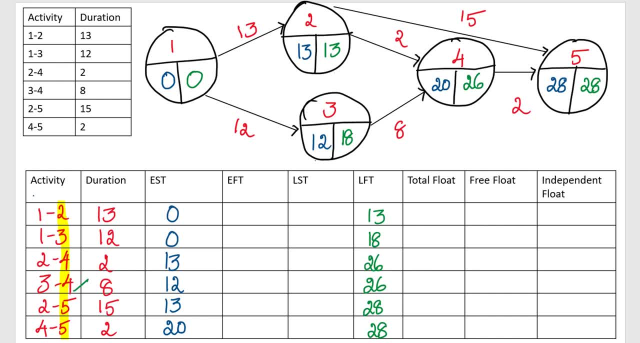 let's calculate eft. now for calculating eft, the formula, what we are going to use it plus duration. we are going to take it so which means 0 plus 13, 0 plus 12, 13 plus 2, and it goes on. 0 plus 13 is 13, 0 plus 12 is 12, 13 plus 2 is 15, 12 plus 8 is 20. 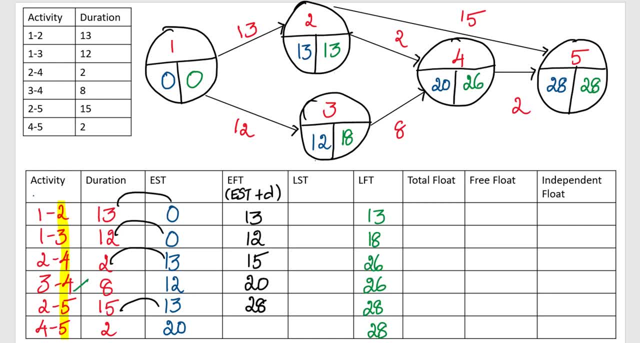 13 plus 15 is 28, 20 plus 2 is 22. in order to calculate LSD, we need a lefty minus duration, so which means you will be taking out this value and subtracting from the duration value. this is what we will be doing. it in other term, subtract. 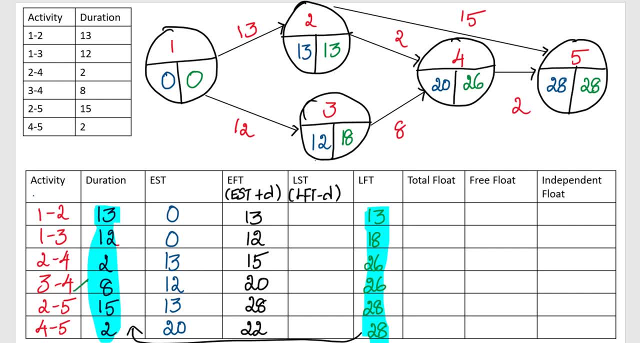 the values of this one with this one. so 13 minus 13, we are going to subtract from the duration value. this is what we will be doing it. in other term, subtract the values of this one with this one. so 13 minus 13, we will have 0, 18. 18 minus 12, we will have 6 here. 26 minus 2, we will have 24- 26. 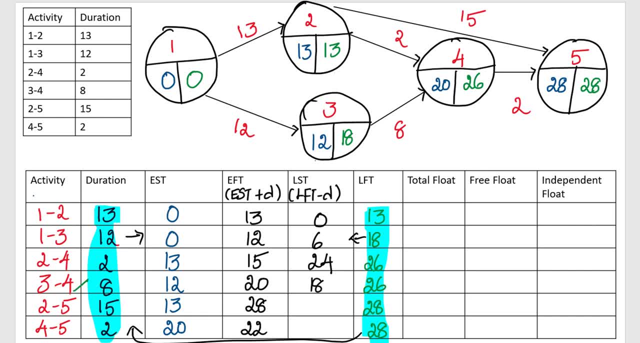 minus 8, we will have 18. 28 minus 15, we will have 13. 28 minus 2, we will have 26. here let's move on to the total float calculation. now for calculating the total float, you have two different ways to do it. one: you can take LFT minus EFT, or you can 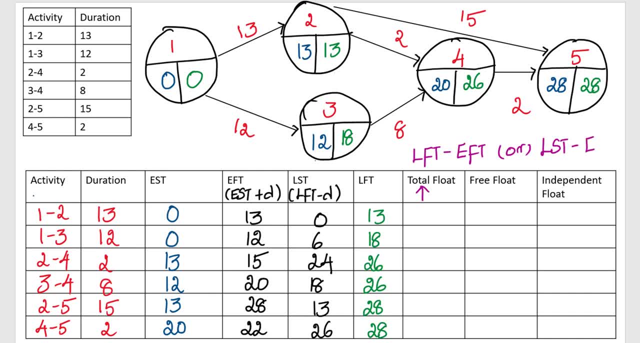 take LST minus EST. so whichever way you go, you should have the same answer. say for example here: 13, 13, 0, again 0 minus 0, it's going to be 0, 18, 12. we will have 6, 6 minus. 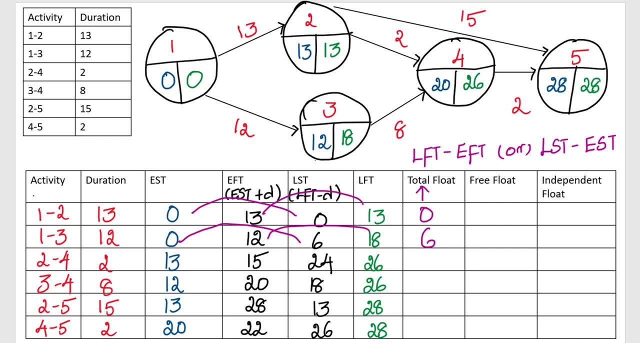 we will have 6 again, 26 minus 15. we will have 11 or 24 minus 13. you are going to have 11, 26 minus 26, 18 minus 12. we will have 6 again. now, 28 minus 28 is 0, 13. 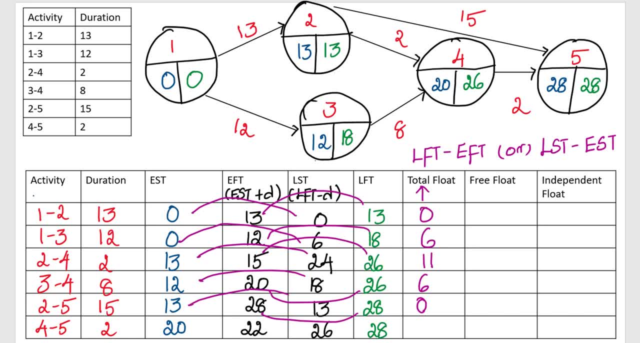 minus 13, again at 0, 28 minus 22, H 6, 26 minus 20, again H 6. at the next level we have to calculate free float. so for calculating the free float we need require a formula even before that, at wherever this color is there, just mark. 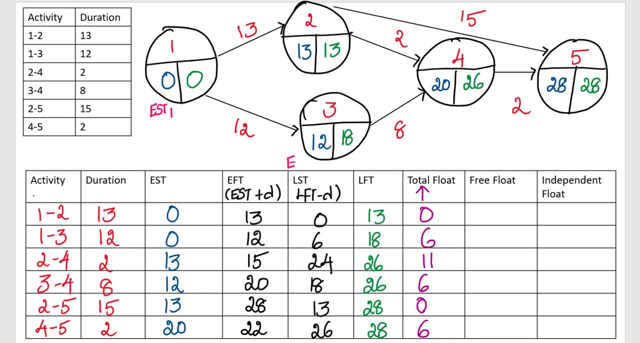 it as ESD one and here its ESD to: here ESD three, here ESD two, here ESD three, here ESD two and here ESD three, here ESD two and here, yes, 3 more. say this value of quarter unit double root. holy picture 2j whether. 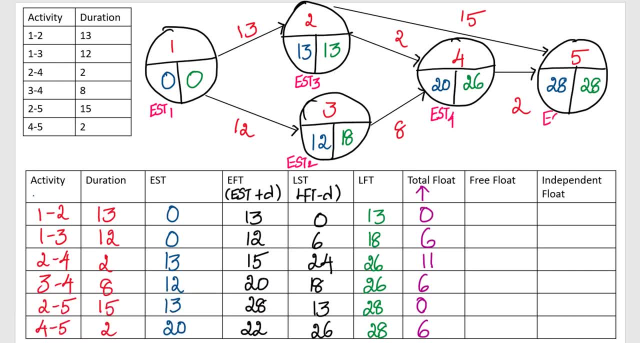 and here we will have will be the whole. we will remember this future zero and ESD4 and here ESD5.. Wherever the duration is there, mark it according to the node. This is D12. duration of 12.. This is duration of 13.. This is duration of 24.. This is duration of 34.. 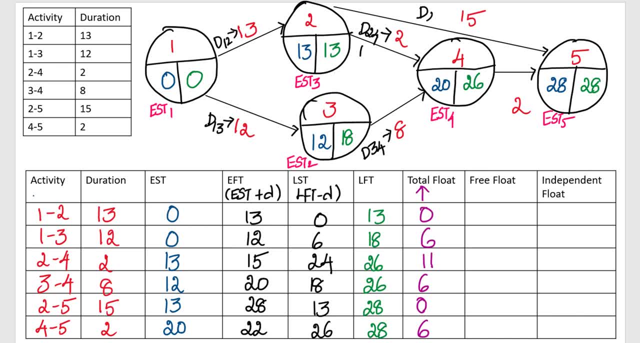 This is duration of 25 and this is duration of 45.. Now let's go to the free float formula. Free float equal to, let's say, for 1-2 activity, EST of 2 minus EST of 1, minus duration of 1-2.. 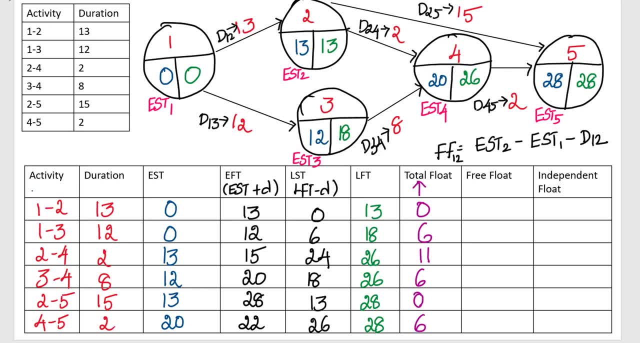 Let's calculate the free float for the first activity. The first activity is 1-2.. So the EST is 13 minus 0 minus 13.. So which means 13 minus 0 minus 13, we will have So which becomes 0. now Let's do it for the activity 1-2-3 also. 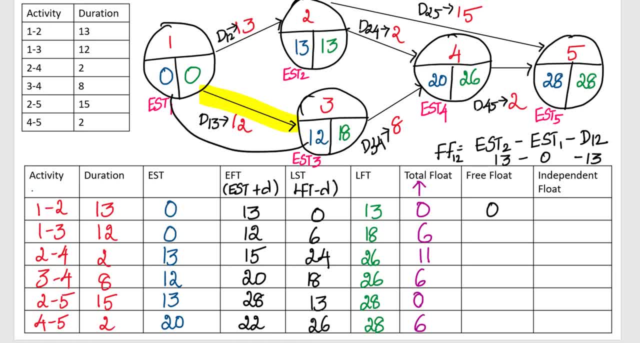 12 minus 0.. 12 minus 0, we will have 12.. Then 12 minus 12, we will have 0 here. So let me write it here: So 12 minus 0 minus 12, we will still have 0 here. 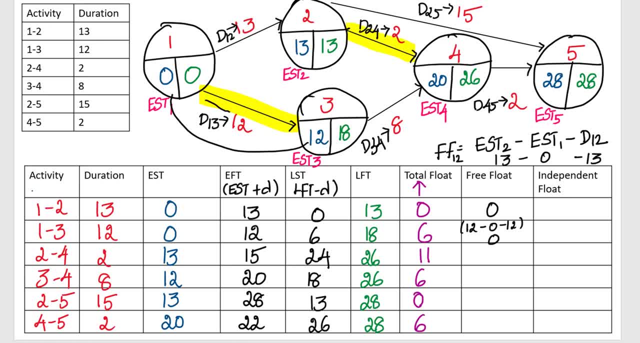 For the activity 2-4, we are going to have 20 minus 13 minus 2.. We will have 5 here. Let's do it for 3-4.. 3-4 is here 20 minus 12 minus 8.. 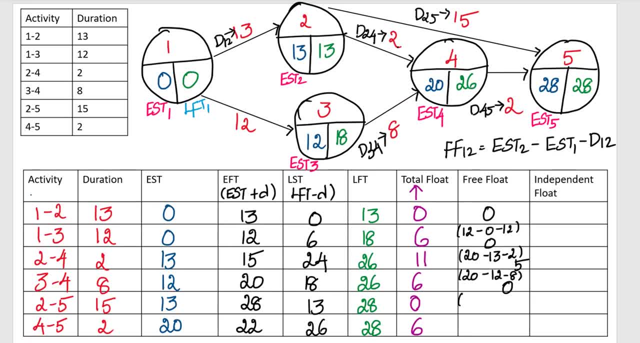 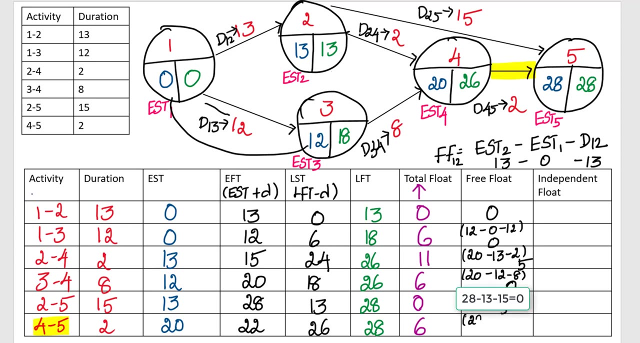 Which will give us a result of 0.. Now let's calculate the free float for 2-5.. The EST of 5th activity is 28 and the EST of the second one is 13 minus the duration of 15, which will give us 0.. Let's do it for 4-5.. 4-5 is here 28 minus 20 minus 2.. We will have 6 here. 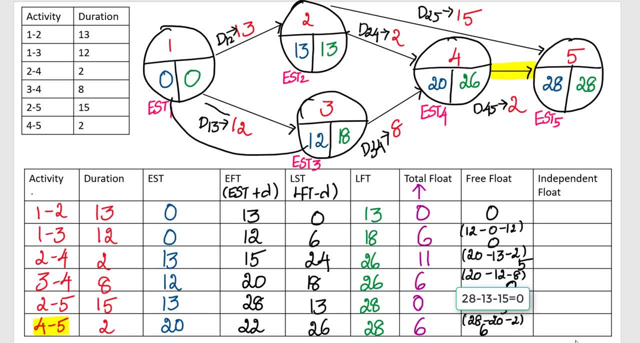 I am sure this is easy to follow. For the calculation of independent float for the activity 1-2-2, the formula is EST: early start time of the second activity minus late finish of the first activity, minus the duration of 1-2.. In order to do this now let's label the LFT also. This is LFT 1,- LFT 2,. LFT 3, LFT 4, LFT 5, LFT 6, LFT 7, LFT 8, LFT 9, LFT 10, LFT 11, LFT 12, LFT 12, LFT 12, LFT 13,, LFT 13,, LFT 13,, LFT 14, LFT 14, LFT 15.. 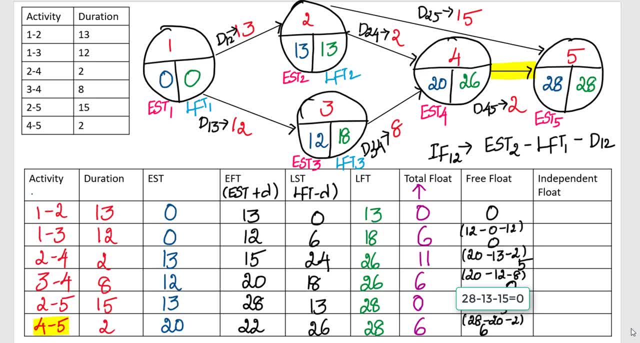 This is LFT 4 and this is LFT 5.. Now for the activity 1-2.. So for EST 2, EST 2 is here: 13 minus 0 LFT 1.. So 13 minus 0, minus the duration here, So minus 13, which will give us 0.. 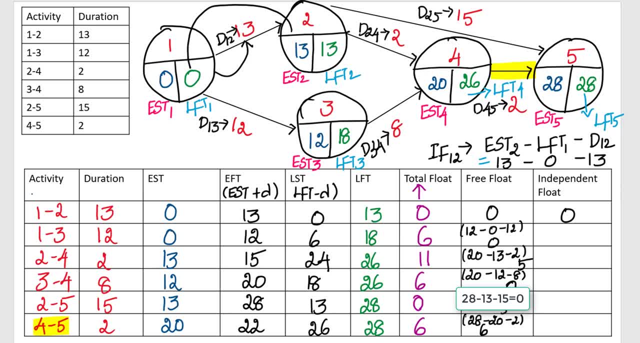 In the same way. let's do it for 1-2-3 also. This is 1-2-3 now. So for the 1-2-3, the duration is: EST is 12 minus LFT. 1 is 0 minus 12, which will give us 0 again. Let's do it for 2-2-4.. 2-2-4, the EST is 20.